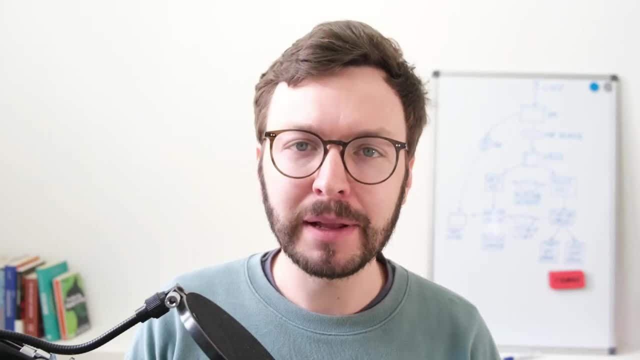 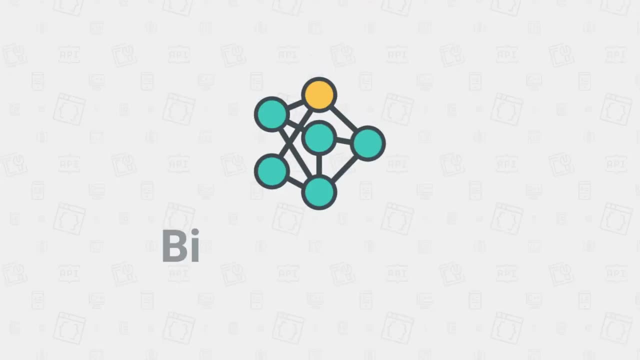 patterns and today we're going to look at the iconic main replica pattern and ask: how does it work and, even more interesting, how does it scale? Let's start from the very beginning to better understand the underlying problem. Imagine you just have set up a database instance on your 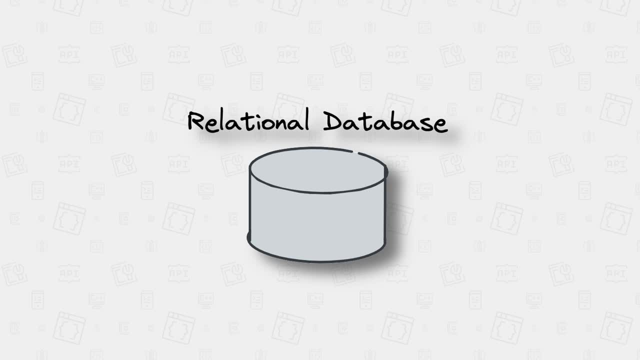 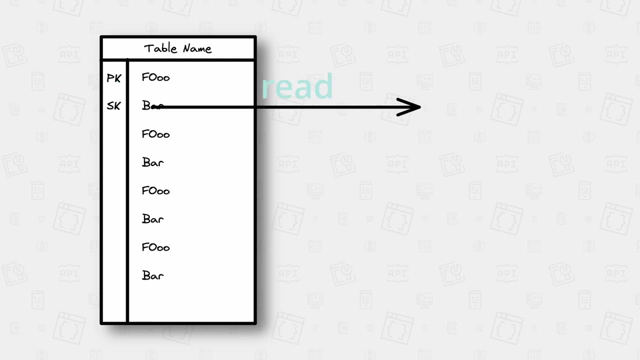 local machine. It already meets all functional requirements you would also need in a large-scale system. For example, you can create the tables you need and you can already read and write from and to them. Really the full story. However, we really didn't waste any time on. anticipating any kind of failure, But you need to know failure is inevitably when you run a large deployment. It's not a question if servers fail, but when and how often they will fail. As a system designer, it's your task to anticipate failures and prevent them from taking the whole system down. Just imagine it's two weeks before Christmas. 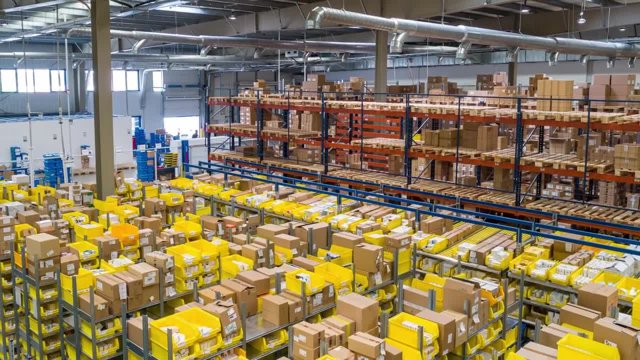 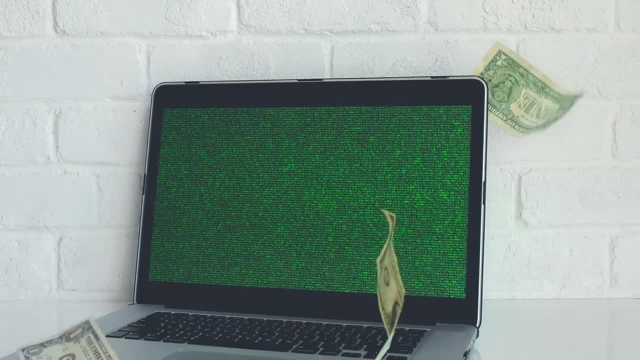 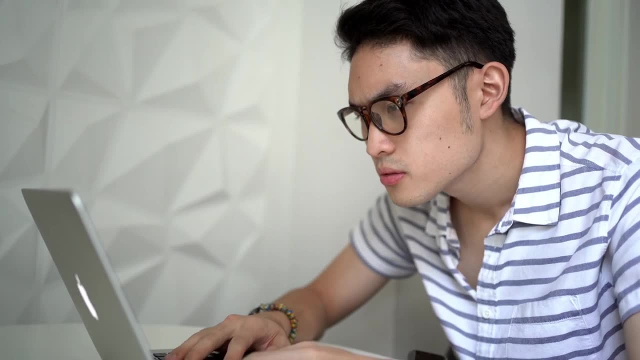 you work for a large e-commerce company and someone pushes a buggy software update to all your databases Due to your naive design, the whole system crashes. You can imagine the revenue loss created by the hours it takes you to get the system back online is well, a lot more than five. 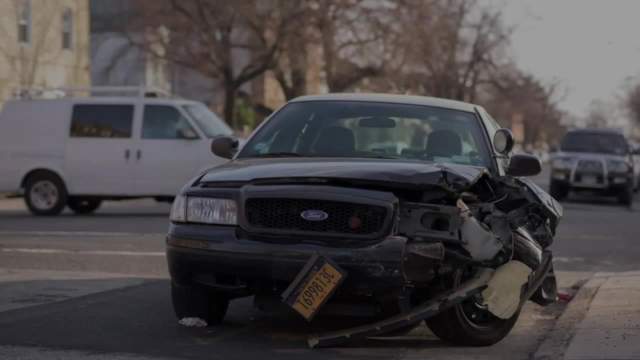 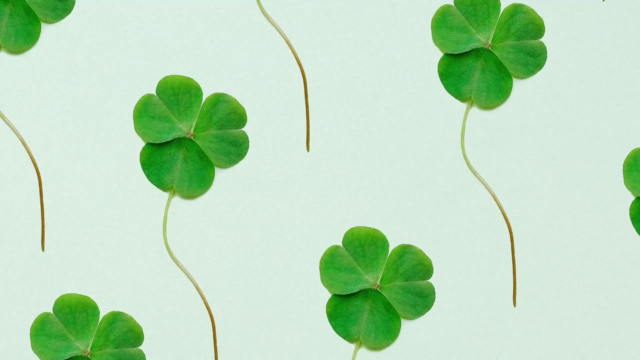 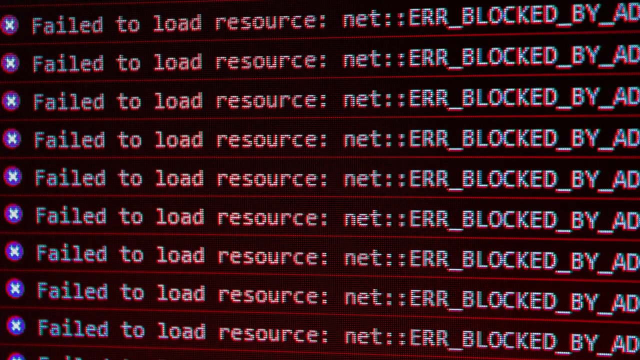 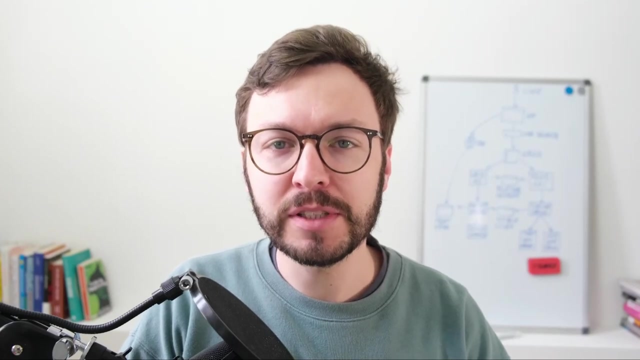 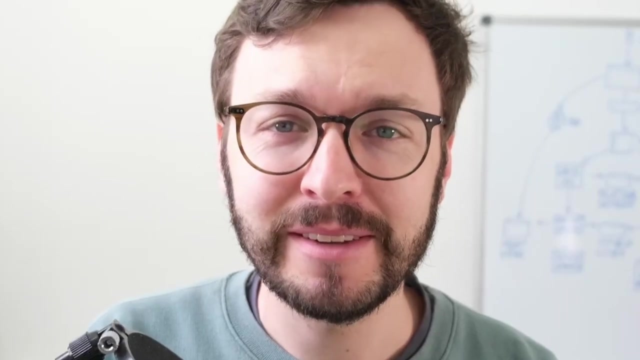 times your annual salary. It's really like designing a car without crumble zones. These areas are engineered to protect passengers by three years, So it's really easy to get to them, and you can even create a lot of design changes by failing first. With replication, you can create similar safe failure modes that 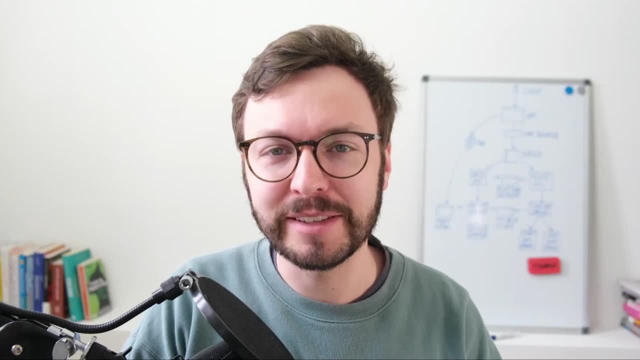 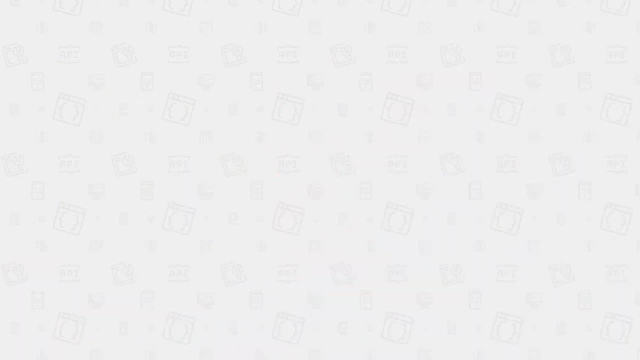 contain the damage and protect the rest of the system. Put simply, replication is nothing else, but lot of problems appear. you need really good answers to, For example, you need to think about in which way you synchronize the different copies. This question is closely coupled with another. 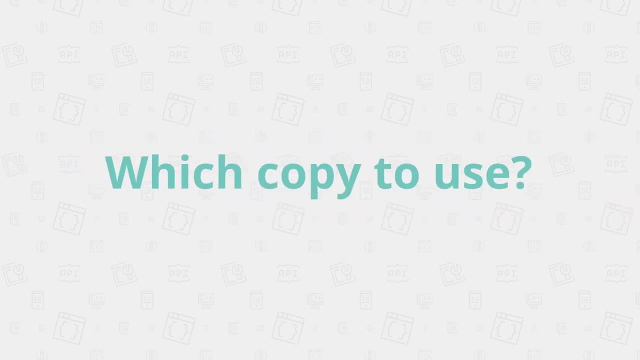 question how users are supposed to interact with a different database service now, which ones are used to read and which ones are used to write. And well, how do we make sure our users always read the latest data and not read from an outdated copy? And 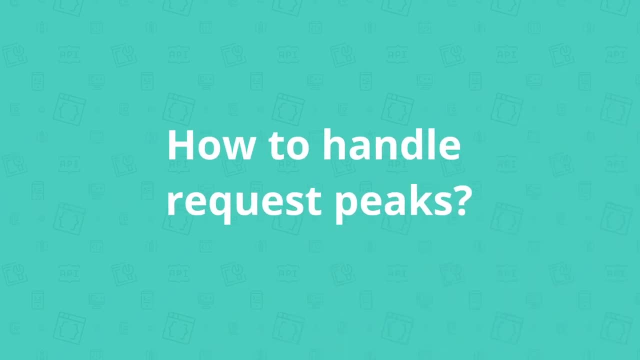 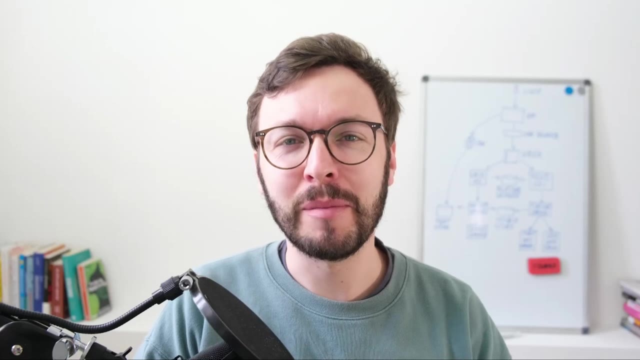 another one is: what happens when there is a peak in requests. Let's say it's Black Friday or just before Christmas. Don't worry, you don't have to come up with answers to those questions all yourself. Engineers have been thinking about them since. 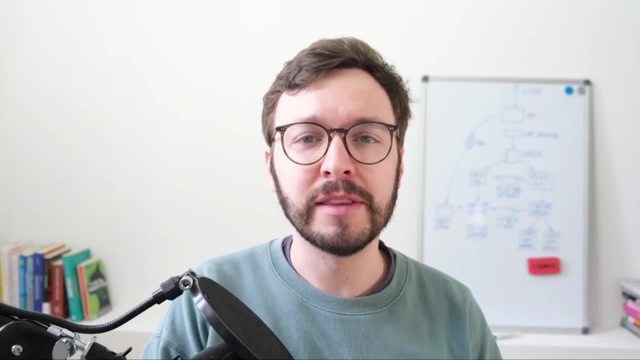 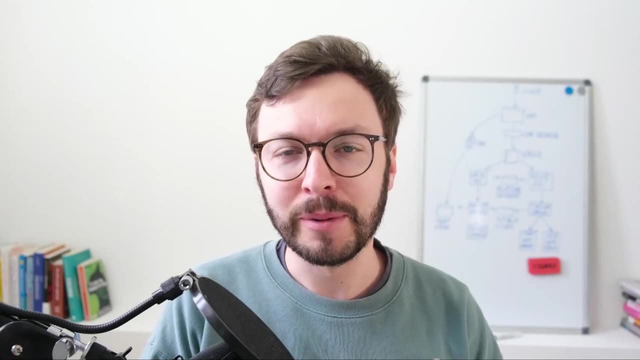 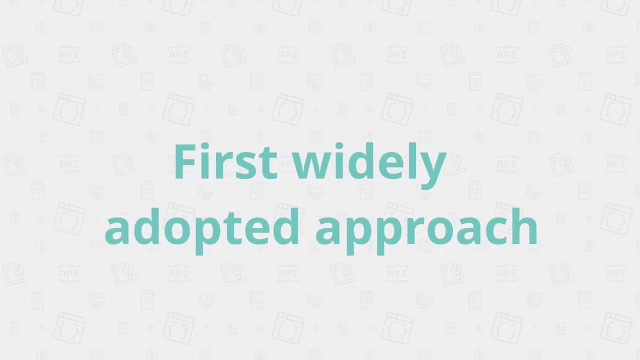 the very beginning of relational databases, And the best of the answers are distilled into design patterns we still know today. The main replica pattern is one of them, So let's discuss it and see what kind of answers it gives us. Historically, the main replica pattern was the first widely 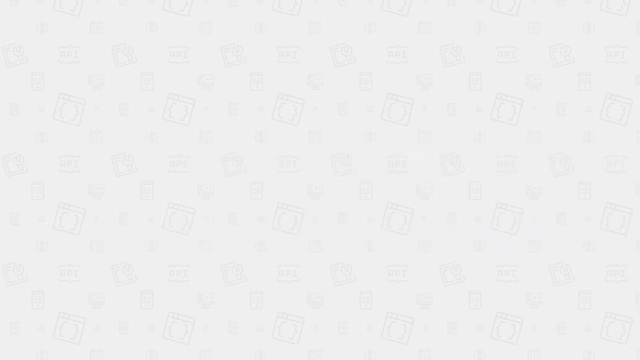 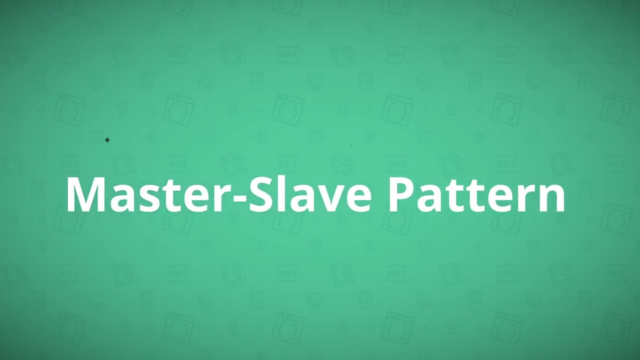 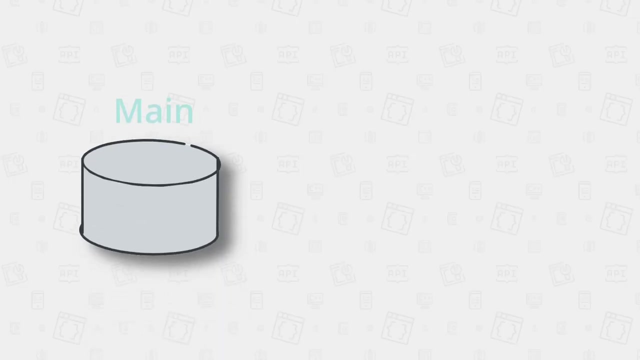 adopted approach to leverage replication to improve the availability and fault tolerance of relational databases. For a long time the term master slave pattern was common. In recent years this terminology has been phased out for good. In fact, there are two types of database nodes. One is called main, the 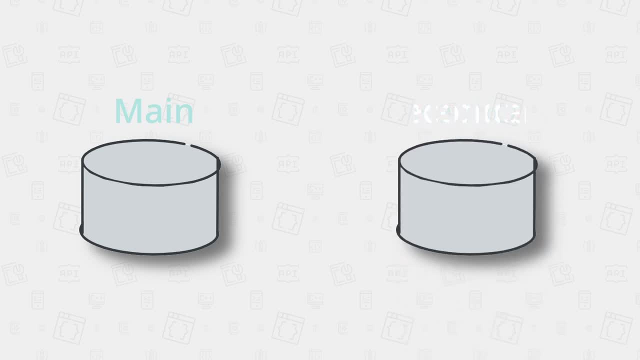 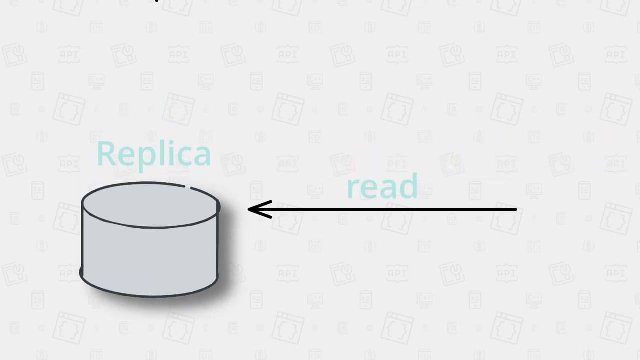 other one is called replica. Sometimes you also hear the terms main and secondary. The main accepts read requests, but it's also the only node in the cluster that accepts write requests. The other replica nodes only serve reads and replicate the latest changes written to the main Typically. 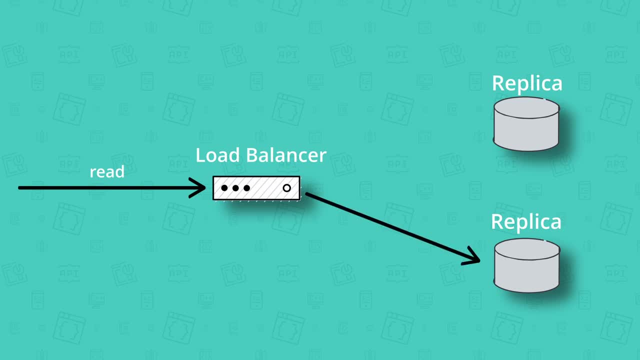 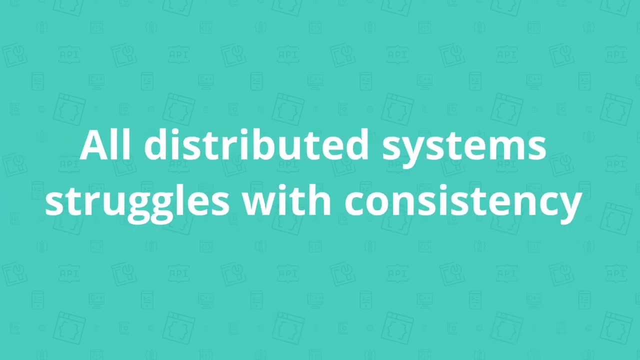 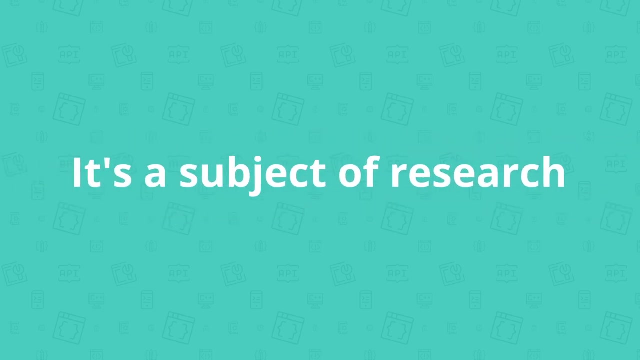 a load balancer is added to the system to route the read requests to the different replica nodes. Just like any distributed system, databases cannot escape the problem of consistency. It's a whole subject of research by itself to keep data across different nodes synchronized. 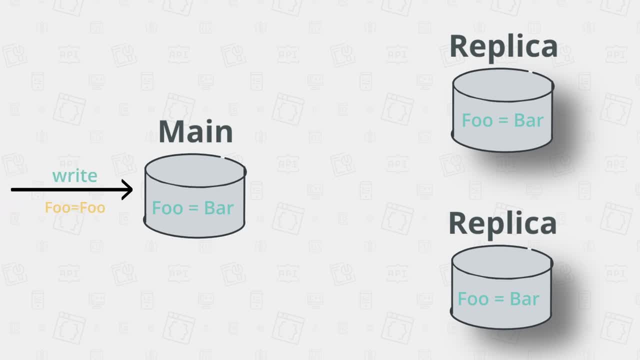 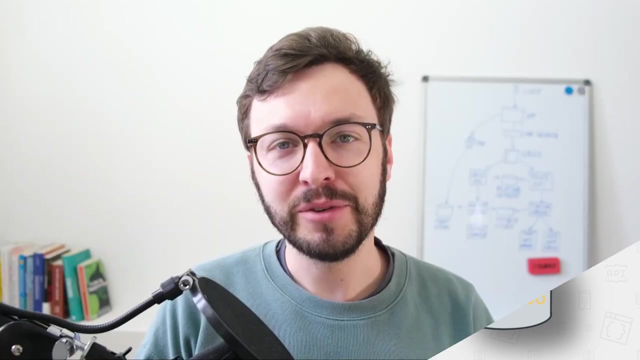 In the main replica pattern, replication of newly written data happens asynchronously. This means that the data on the main and the replicas may be not consistent for a while because replicas haven't caught up with the latest changes yet- If you need a fancy term to describe this phenomenon- in your system design interview. 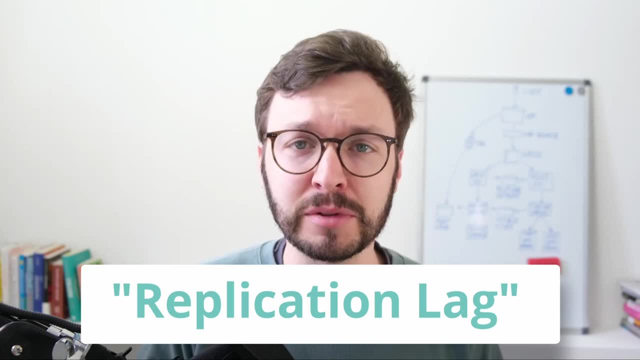 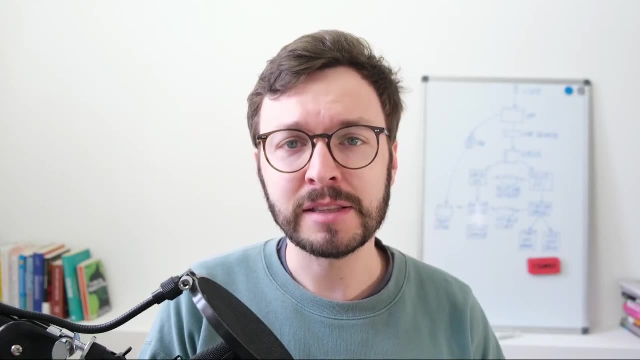 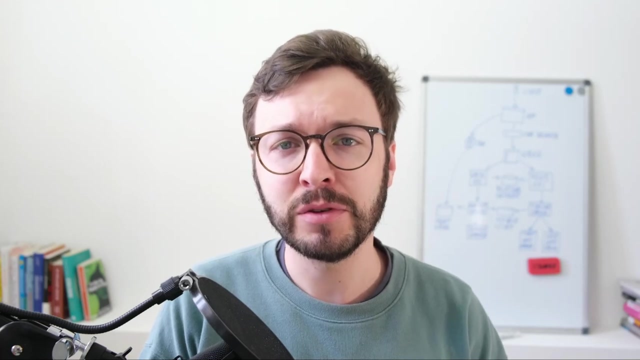 you should call it replication lag. The consequence of those lags is that your relational database, which applies the main replica pattern, has the property of eventual consistency. It's not strongly consistent And this is a big difference And, depending on the use case, this can be critical. However, there is an 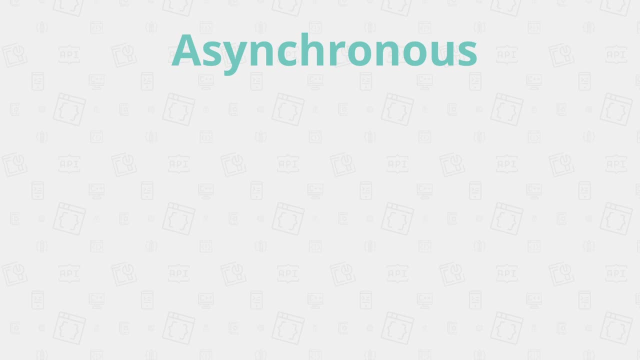 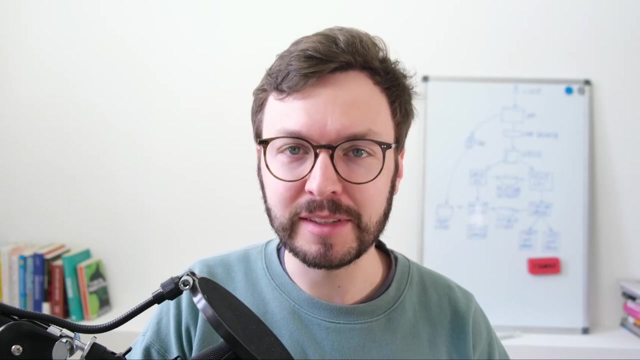 intriguing advantage of using asynchronous replication: It's much faster and scales better than synchronous replication. There's also a middle ground solution called semi synchronous replication. If you want to learn more about the different replication methods, I have a dedicated video on this topic and you'll find a link to. 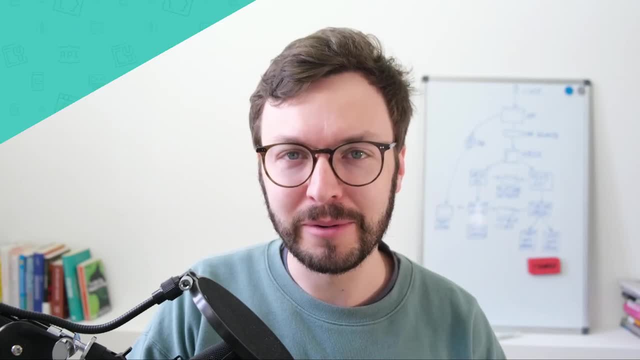 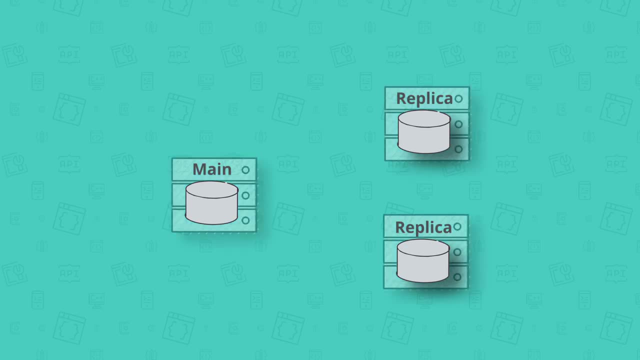 it in the top right corner or in the video description below. In a typical setup you would distribute the nodes over different physical service enclosed geographical proximity, most likely within the same data center. That way you reduce the impact of hardware failure, But still you can keep. 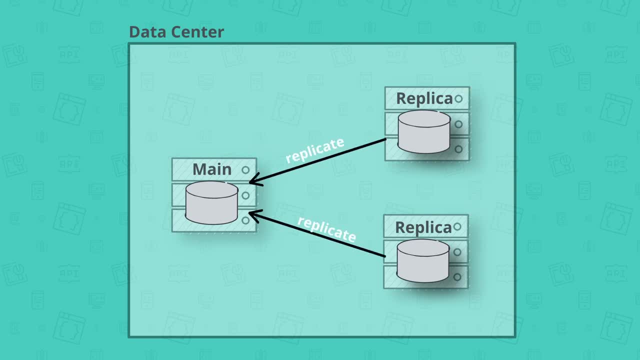 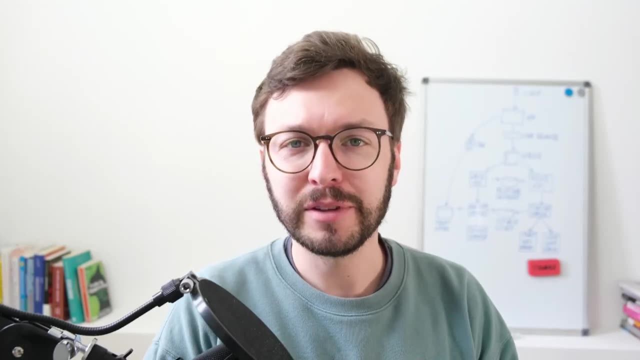 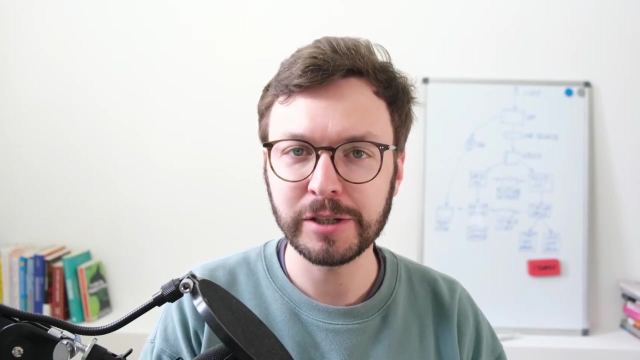 the latency relatively low. Otherwise, your design might come with a replication lag and grain to it, even though there isn't even load on the system yet. Now, after we worked through the basics, I want to show you a couple of failure scenarios So you better understand how this replication 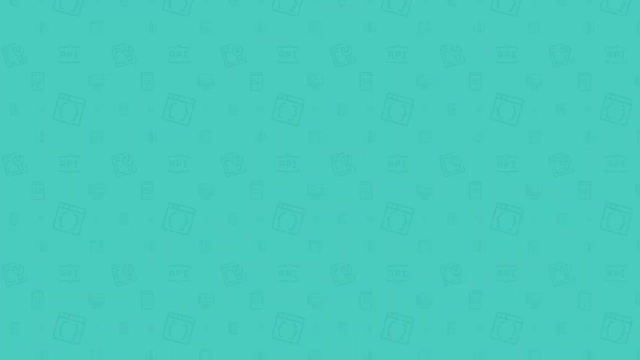 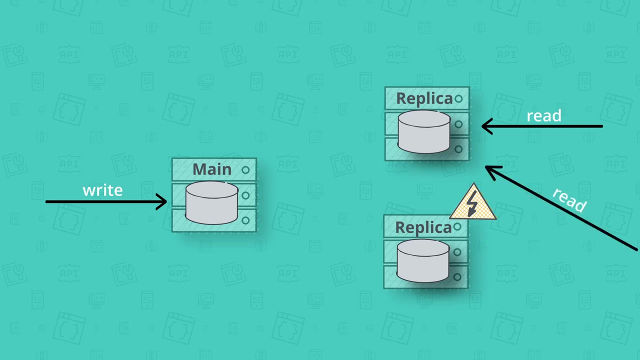 pattern works in critical situations. Let's start with the case that a replica node crashes. What happens then? I give you a moment to think about it. Well, not a lot, In fact. the traffic that would have been served by the node will be rerouted to other replicas. That increases. 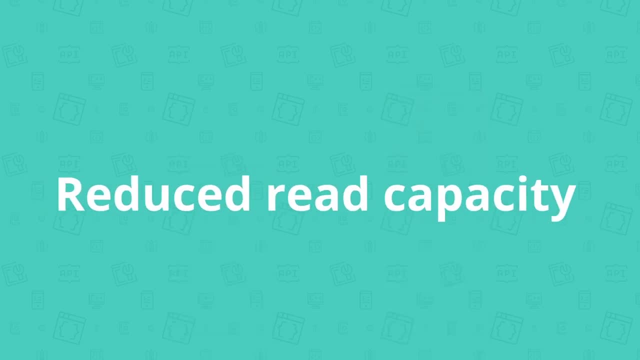 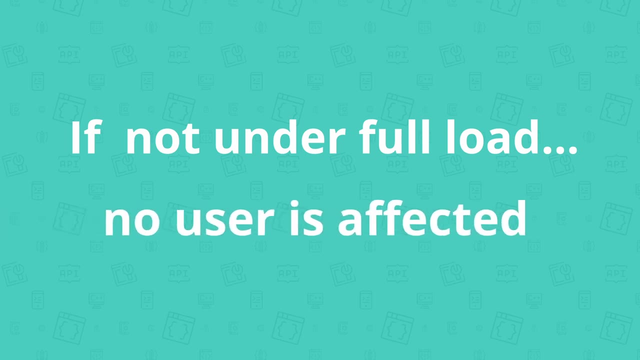 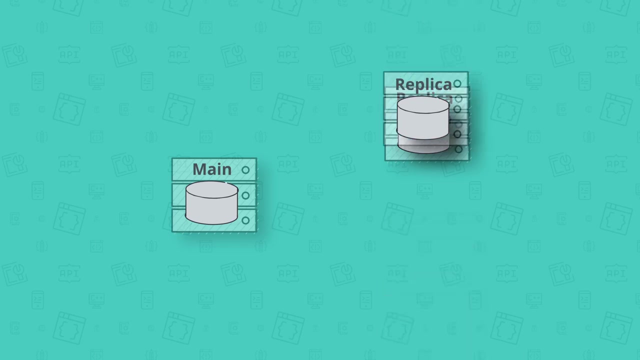 the load of them, The maximum read capacity gets reduced. But as long as the system isn't under full load already, the user isn't affected by this incident at all. The next forward response is to simply spin up a new replica node to replace the faulty one. I say: oh, simply spin up a new. node, But you would actually need a backup- a fairly recent one even- to do that, Because otherwise your new node doesn't know anything about the latest state of the database and would need to replay a lot of events to catch up with the main That. 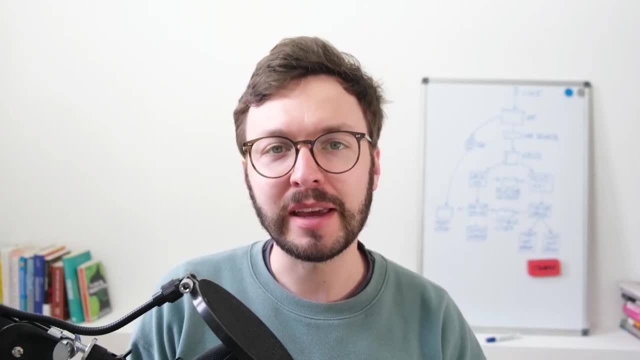 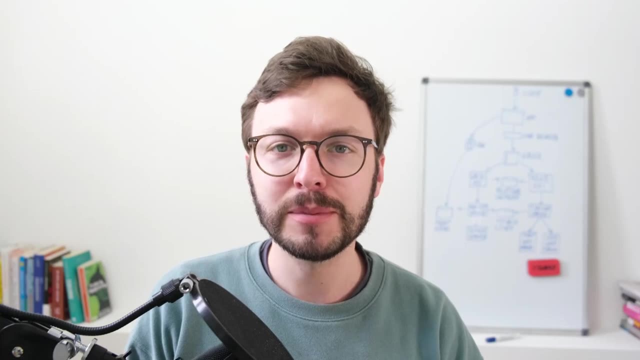 means it would come in with a big replication lag. It would take ages till it actually could replace the faulty node which just went down. If you don't know a lot about backups, don't worry. it's on my backlog and I'm gonna do a video on that. 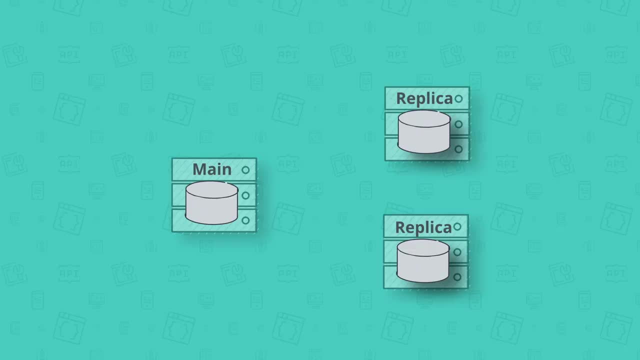 topic as well very soon. Now we get to the most critical situation that can happen: Your one and only main node goes down due to a hardware failure. What can you do about it? Again, I give you a moment to think. First, thanks to replication, the system remains able to serve. 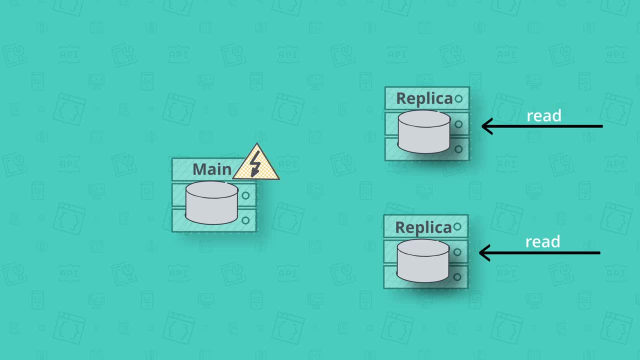 read requests, which is great. But what happens if you don't read the requests? Well, it's not great, as most modern applications are very read intensive. They have a high proportion of reads compared to writes, But the system still lost all abilities to serve write requests, And that's. 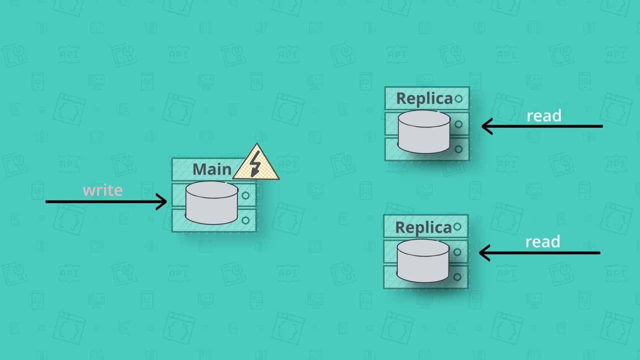 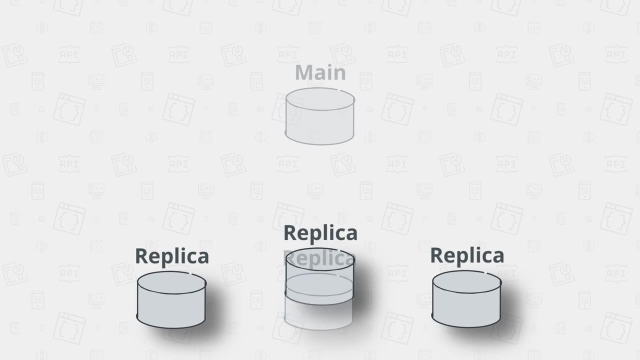 really, really bad because it affects the user experience. So the clock is ticking And the system really urgently needs to get back its capabilities through serve write requests. If you lose your main node in the main replica pattern, you can use replicas to act as the new main and start to accept write. 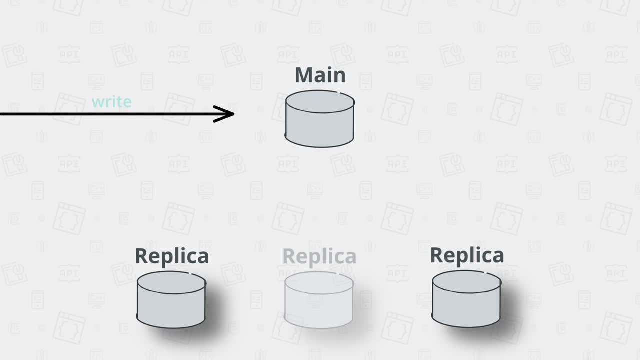 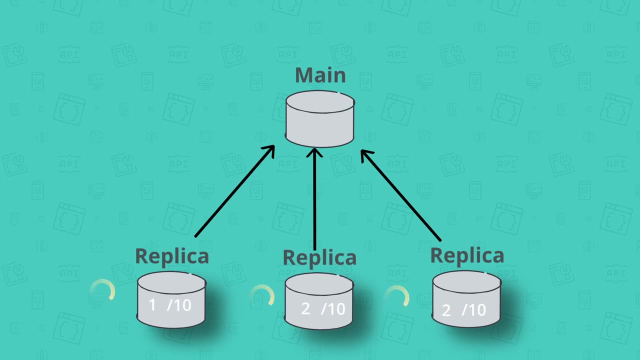 requests. The big question is how to decide which replica should be the new main, Due to the asynchronous nature of replication in the main replica pattern. all replica nodes are in a different stage, replaying the latest changes. Once the main node is down, all of those replays stop. So the most 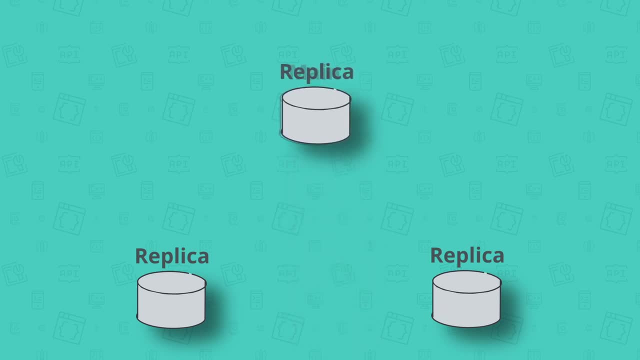 reasonable choice for promotion is the replica that is most up to date. Once promoted, all other replicas need to start replaying the changes. This newly promoted main is ahead of them. As said, the most up to date replica is promoted, as in: 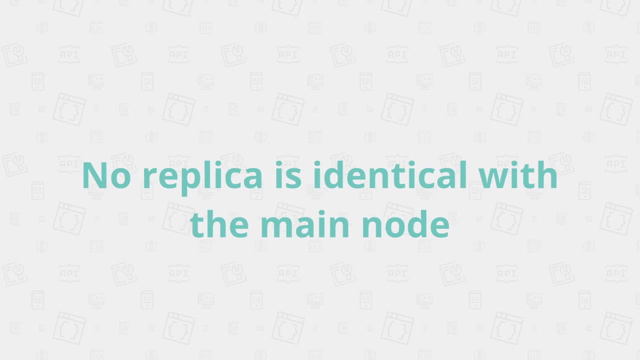 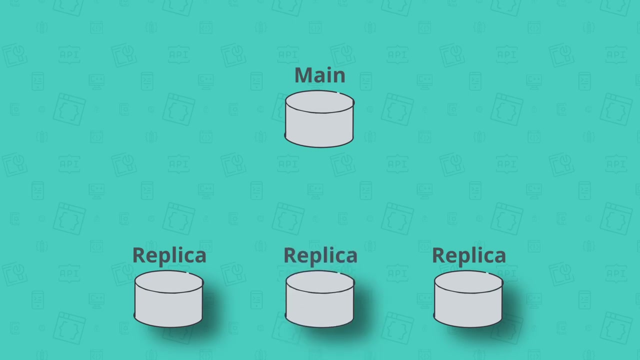 most cases, no replica is actually identical with the main, And that means all data which isn't replicated in the moment the main goes down is lost. Last but not least, to also get back its full read capacity, the system needs to spin up a new replica that. 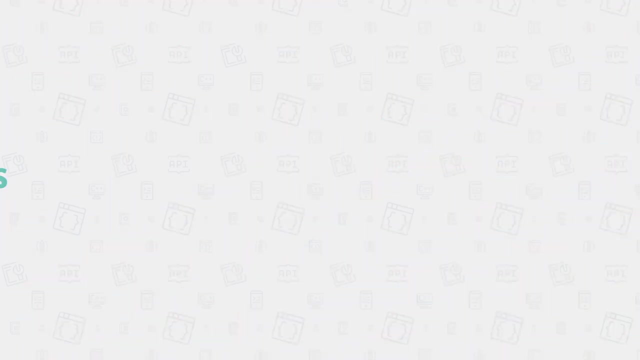 replaces the just promoted one. That's how a replicated database reacts to failure scenarios. It's very straightforward to see how it significantly increases the system's availability, But we're not done yet with exploring the main replica pattern. Availability is just one of the desired properties. a 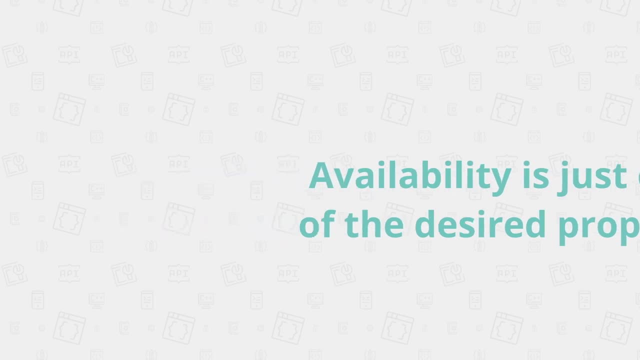 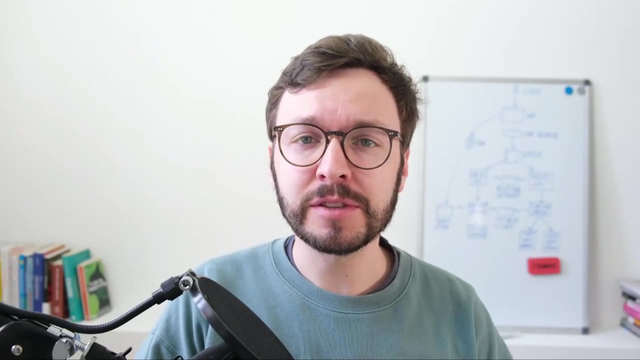 system needs to serve large scale applications. Another crucial one is scalability. Let's investigate which methods you can leverage to tweak your main replica architecture in order to keep up with an ever growing user base. To give you an idea, Netflix just grew their user base to 200 million users. 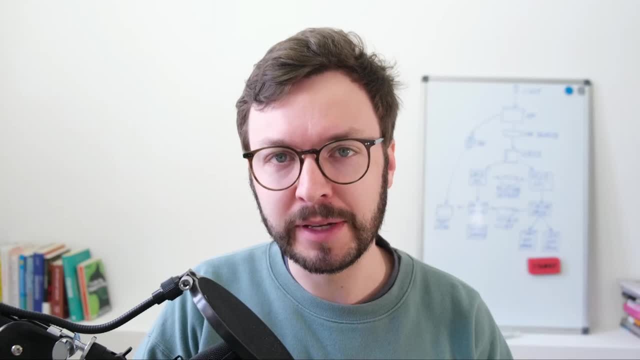 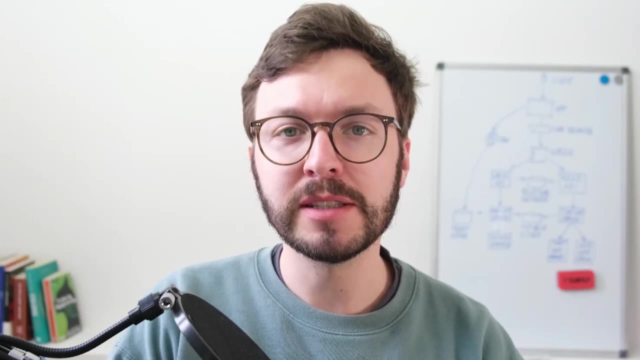 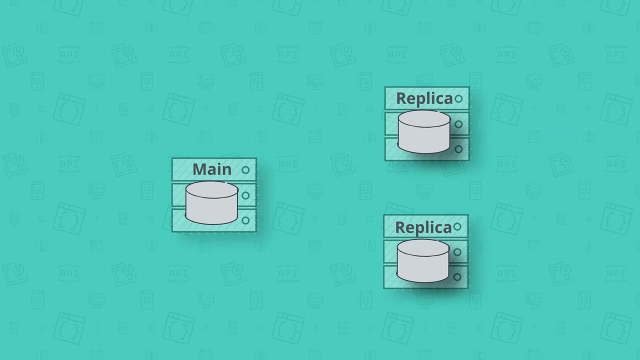 this year. And this is still a small user base compared to other large scale systems like YouTube. What happens if you don't scale your system alongside a growing user base is very simple to explain. First, your replicas get overwhelmed with more and more read requests. At one point, 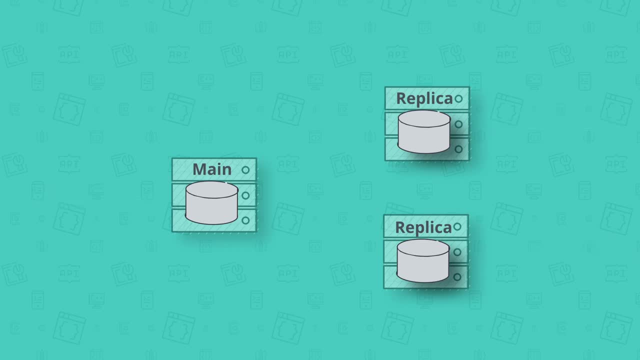 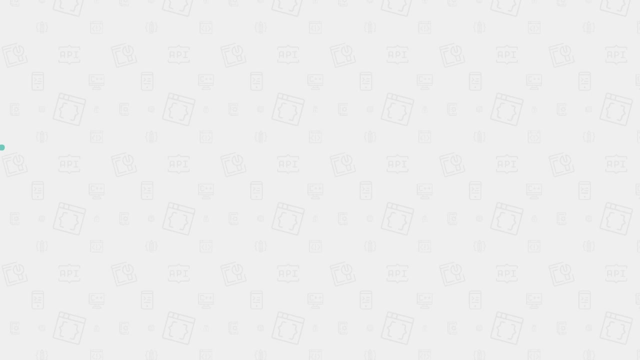 write requests also increase And that means that replicas need to replay more and more writes And they also need to serve more and more read requests. That leads to an increasing replication lag because they simply can't catch up. A massive replication lag again leads to poor user experience, as users are. 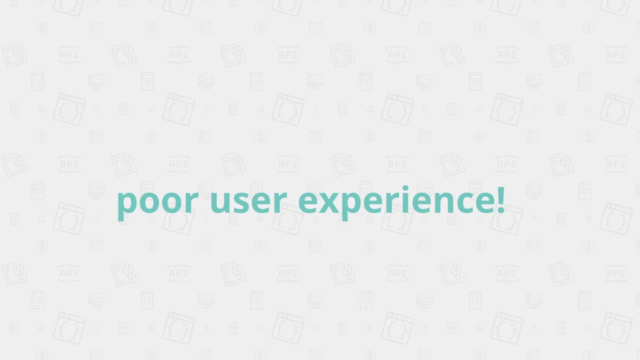 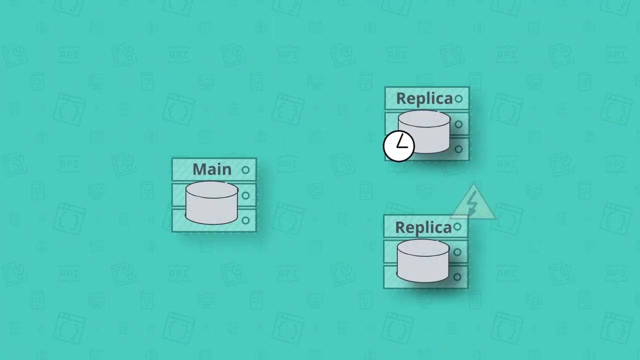 presented with outdated data And it takes increasingly long to actually show the latest changes. Eventually, notes run out of memory and crash, which increases the pressure on the remaining notes And it speeds up the collapse of your whole system. To prevent such a scenario, the system needs to be tuned to be always 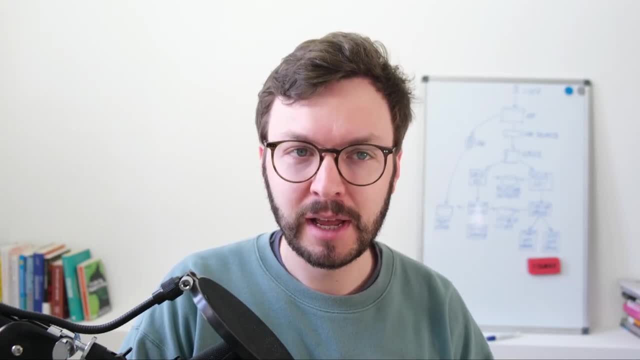 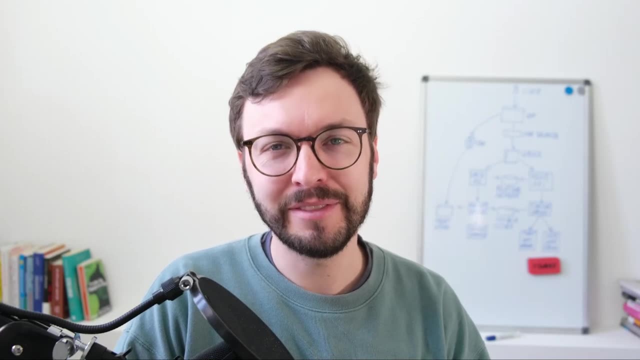 ahead of the increasing read and write requests And you still need a good amount of backup resources to handle peak loads. How do you scale read traffic? I'll give you a hint. This one is the easy one And it's also the reason why the main replica 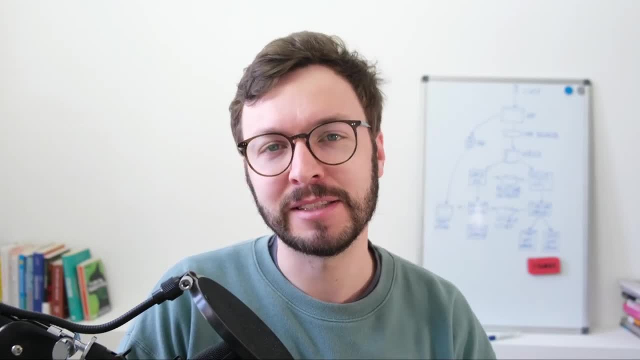 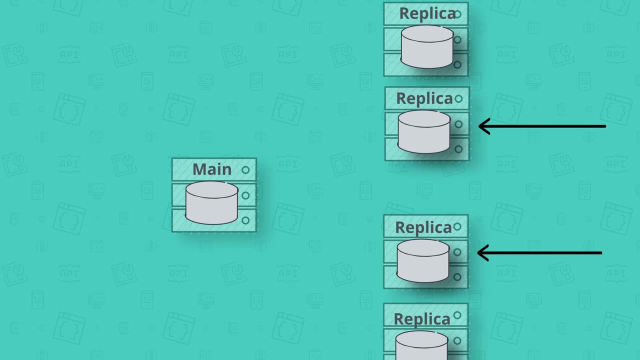 pattern and relational databases have withstand the test of time so well. You simply add more replica notes. Each replica note runs on its own physical server. The fancy term to describe this approach is horizontal scaling. It's great that we can achieve this, because it's a cheap way to. 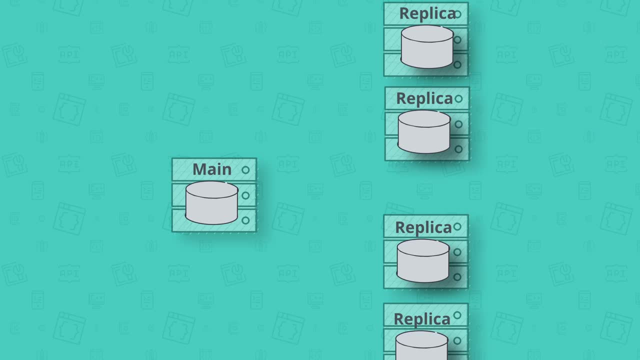 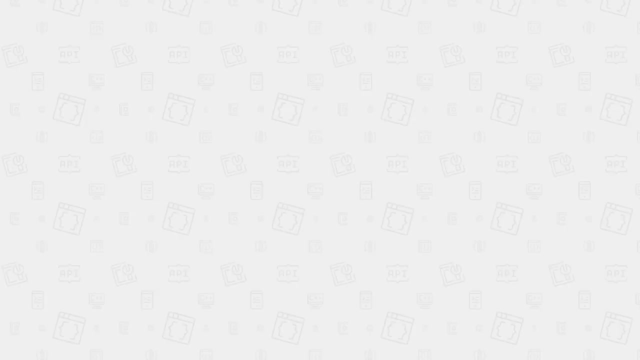 extend the system's read capabilities. Of course, there's also constraints to this approach. As this new replicas need to be synchronized, the network traffic would increase significantly, But that's a story for another video. For now I want to focus on the second, scalability challenge. 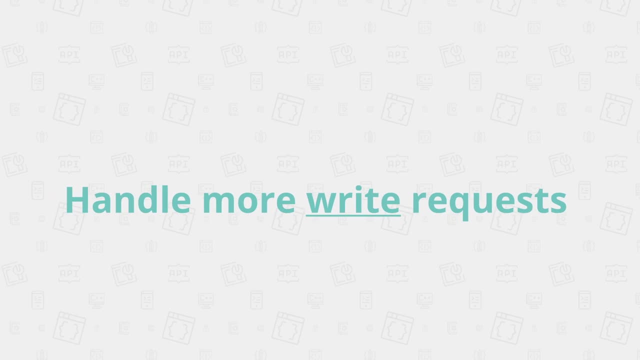 here making the system handle more write requests. And here comes the tricky part. We only have a single main note And while we theoretically can increase the amount of replicas to infinity, the main note remains to be just one. So over time the main note really becomes the bottleneck of the 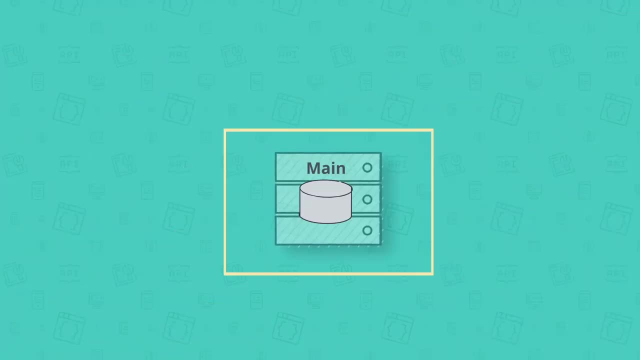 system. What can be done is to increase the hardware capabilities of the physical server. the main note runs on. Again, here's a fancy term, It's called vertical scaling. However, this approach quickly gets to its economical limits Because adding more and more memory and CPU power to a single machine. 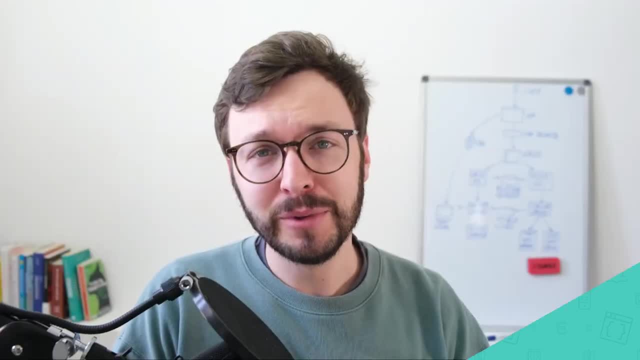 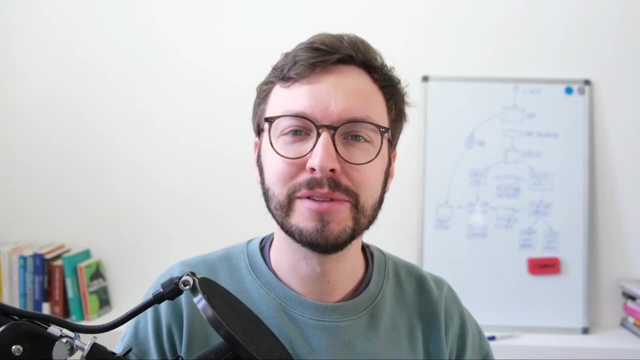 eventually becomes very expensive. If you want to learn more about the different approaches to scaling, you'll find a link in the top right corner to another video of mine and again in the video description below. So there must be another way to scale Write requests, but it's impossible in the main replica. 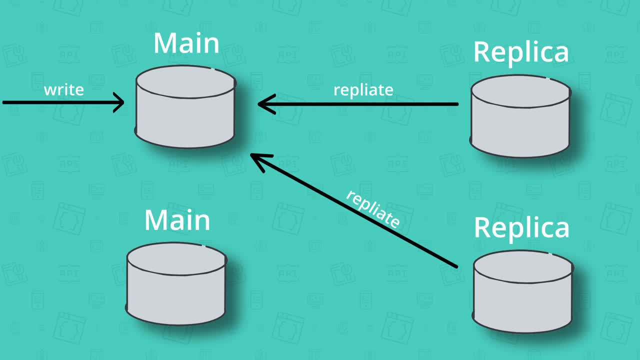 architecture to add a second independent main note. How would you maintain consistency over the system if you would have two nodes that accept writes? But what if we would create multiple fully independent data sets, each of them with their own main and replicas? With this architecture, it's possible to 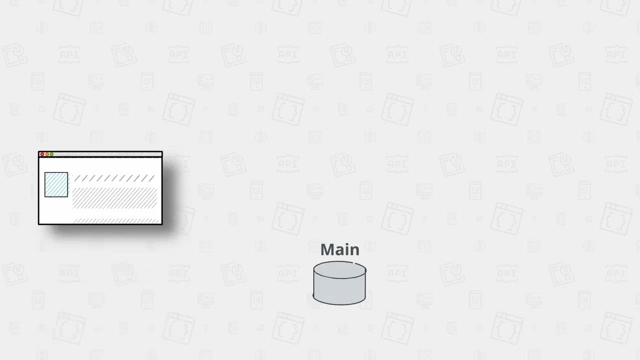 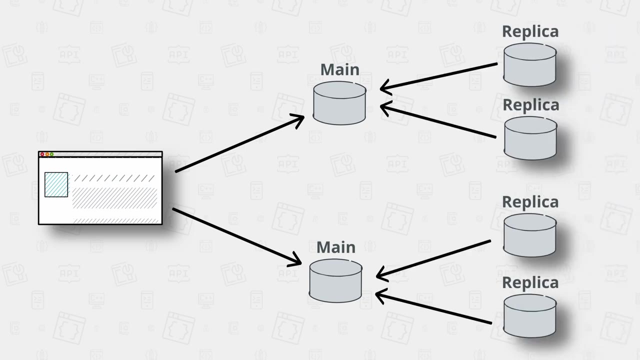 scale write requests. All such requests would need to be directed to the partition. The partition is responsible for the unique subset of data that is intended to be updated. That way, all write traffic can be split up, directed to different independent main nodes. Our 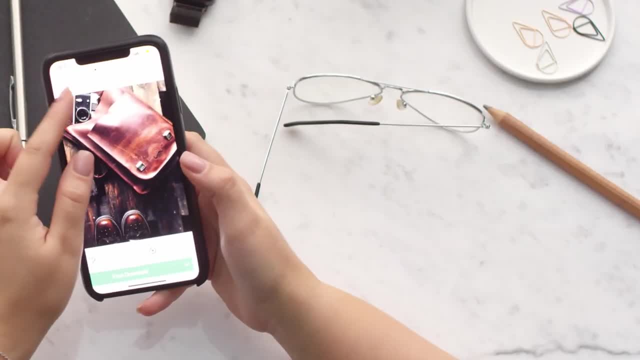 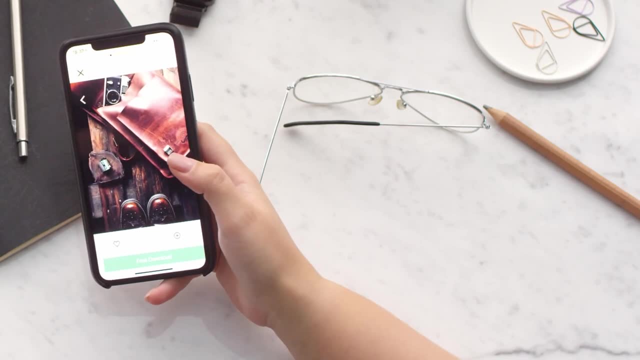 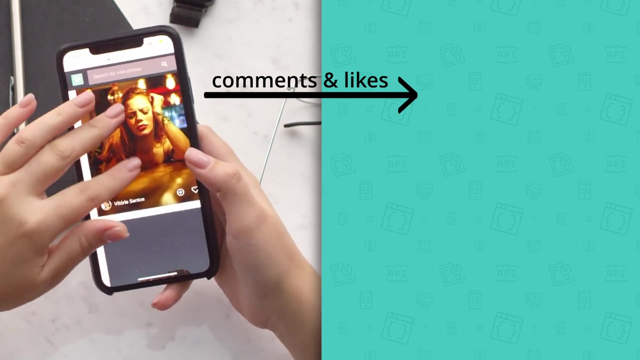 original bottleneck is gone. Let's look at an example. Imagine you have a single large database handling all data of a social media platform like Instagram. You have many write requests as people keep commenting and liking posts, But also posts themselves are write requests. By dedicating one 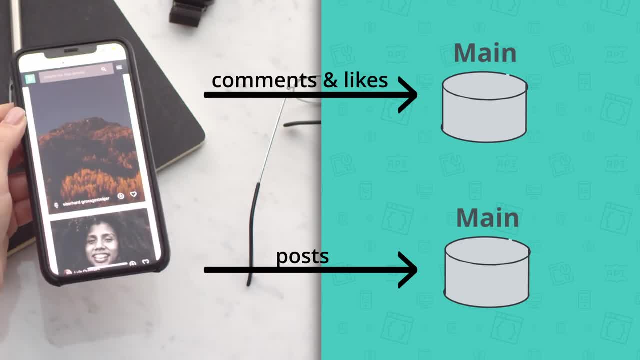 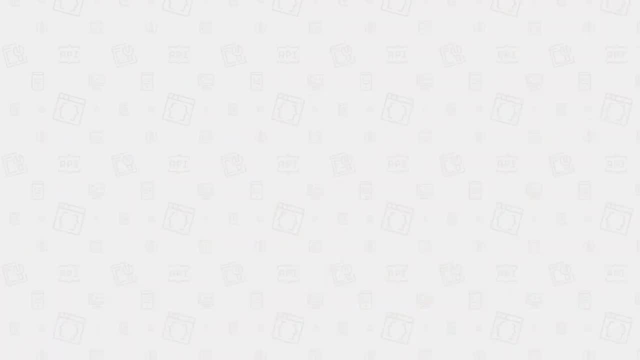 database to only stop comments and likes, while the other one is handling the content of posts. you can reduce the load on each of the main nodes. To describe this approach, people use all kinds of fancy terms. The most common is sharding, But there's 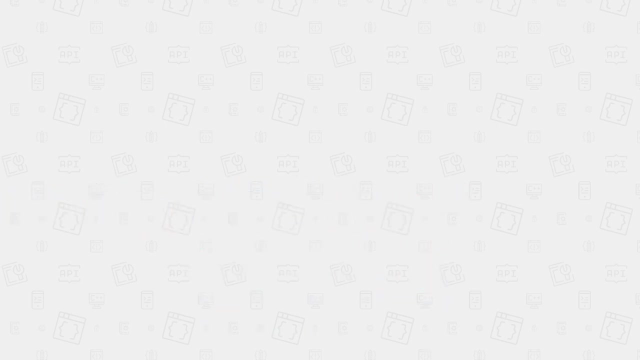 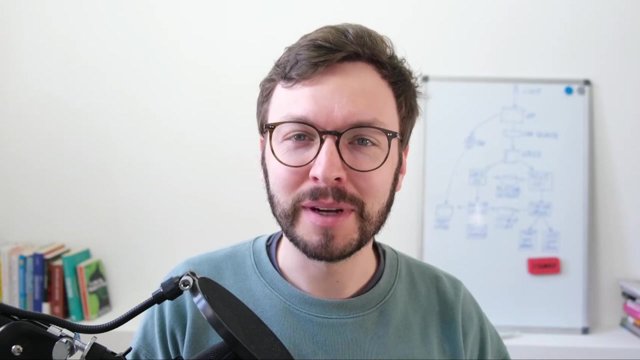 also other names, like splintering or horizontal partitioning. Each partition is also referred to as a shard. For today, there's really nothing else to do but wrapping up all the new concepts and the new fancy terms. you need to speak the same language as. your interviewer in your system design interview. First, database replication is a technique to increase the availability of a database by replicating and distributing the data over multiple nodes. That way, the risk of data loss and downtime due to hardware failure or human error gets reduced. 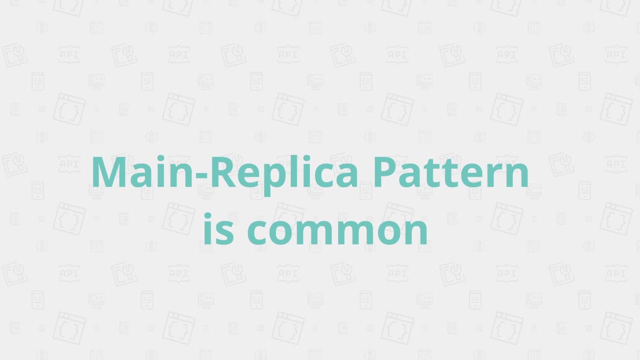 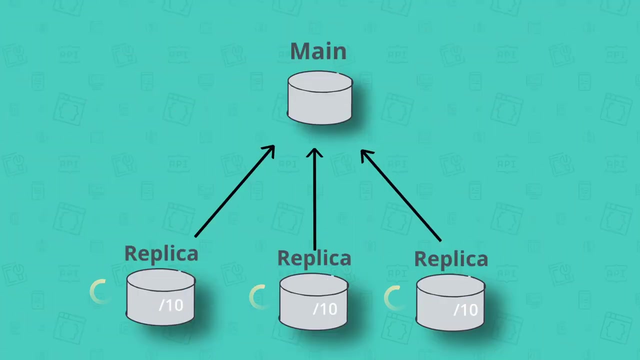 A common replication pattern is the main replica approach. It creates two types of nodes: one single main node that handles write requests, and replica nodes that only handle read requests. The replicas receive the latest data changes made to the main in an asynchronous fashion, And then they try to replay all changes as fast as they can. 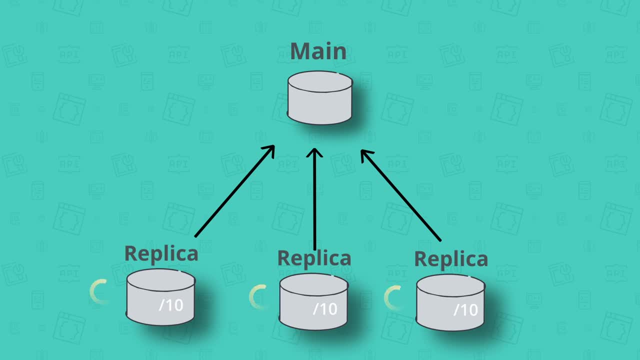 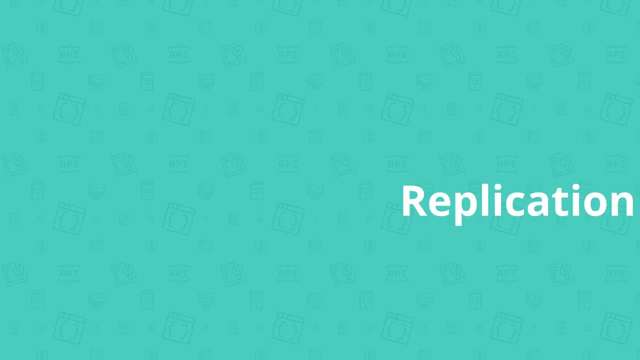 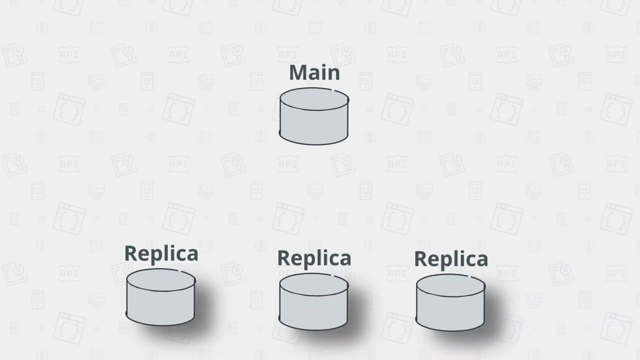 But there will always be an individual replication lag for each replica. That's why the system only can provide eventual consistency. Replication lags become worse with increasing workload and can affect the user experience at one point. In case individual nodes fail, there is 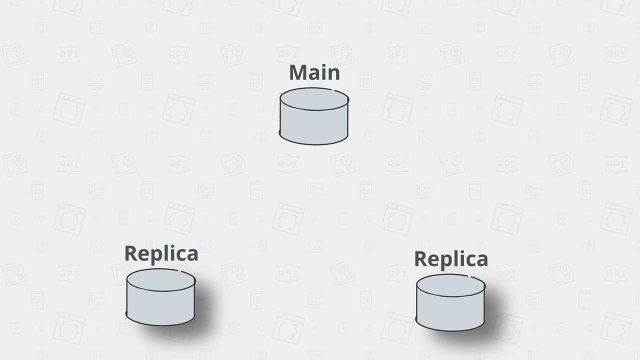 really two options. If a replica fails, simply replace it with a new instance. If the main node fails, the most up to date replica will be promoted to be the new main. Due to asynchronous replication, there's always the risk of data loss. 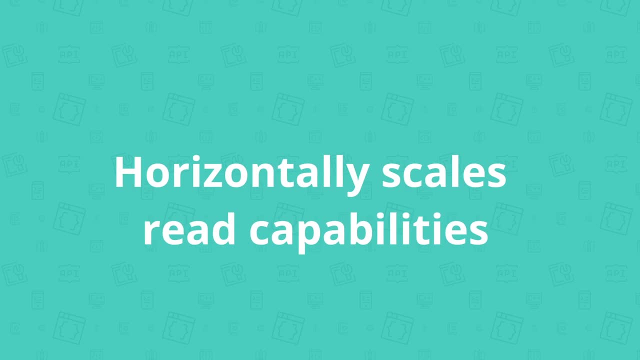 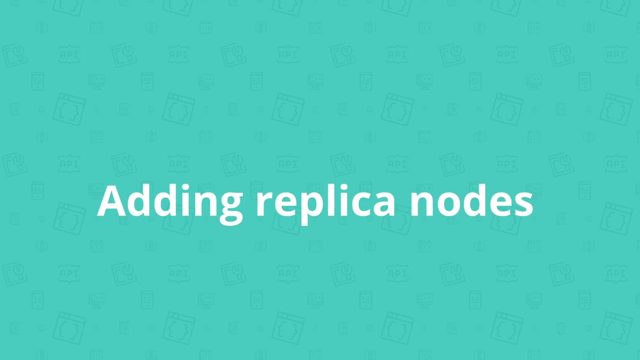 Replication is a great way to horizontally scale the read capabilities of relational databases. by adding more and more replica nodes, It comes at the cost of increased network traffic, though Scaling write capabilities is possible to a certain extent by increasing the memory and CPU power of the physical 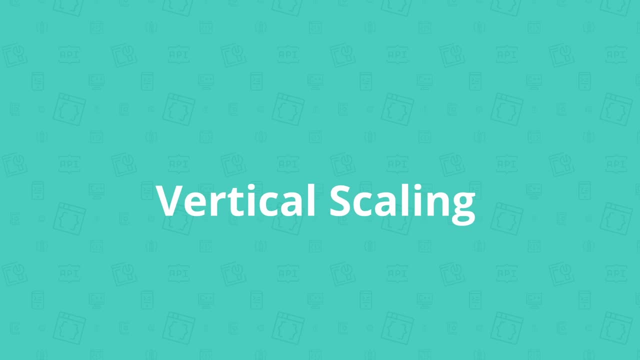 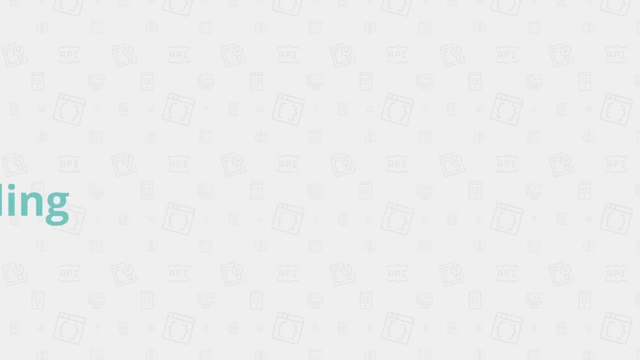 server hosting the main node. That approach is called vertical scaling. Once the economical limit is hit, database sharding is the next best option. Sharding follows the idea of partitioning data into multiple independent databases, called shards, Thereby the load on each. 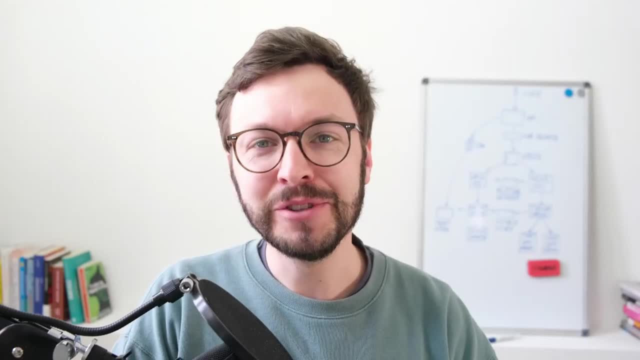 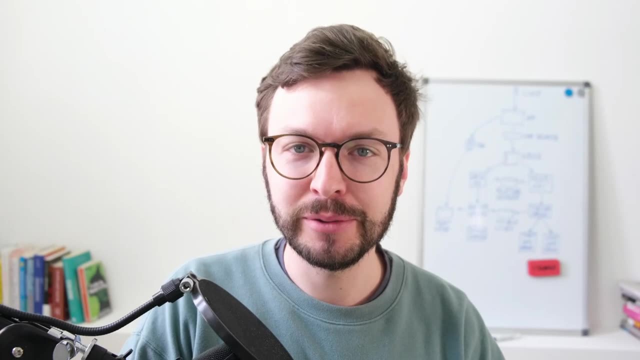 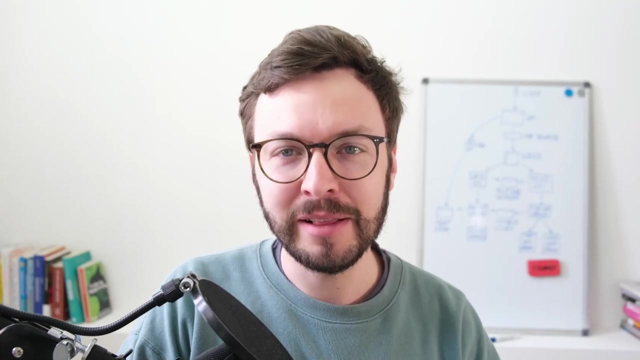 individual main node is reduced. I hope you enjoyed this video as much as I enjoyed creating it. If you want to really deep dive into the preparation for system design interviews, I might can help with that. On this channel, I fully focus on teaching you all the theory you need to nail the 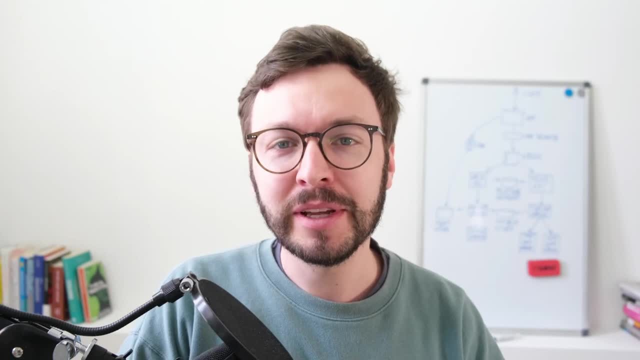 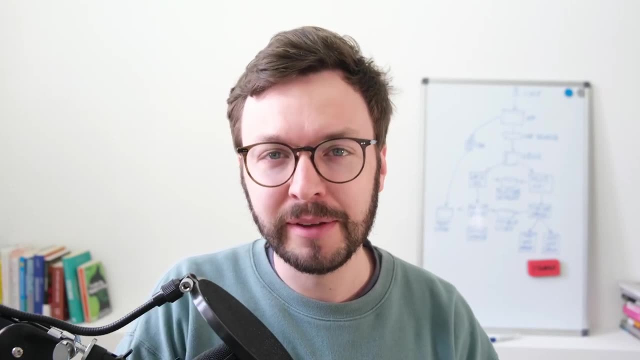 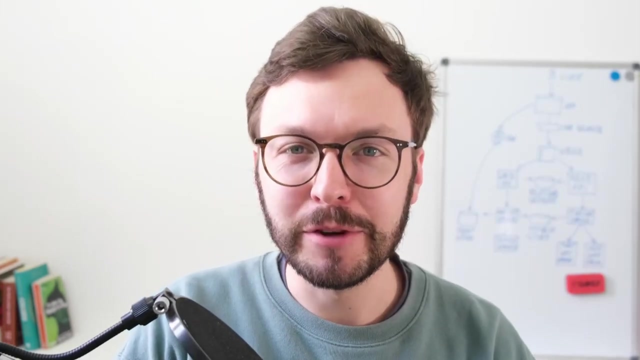 system design interview at any big tech company. You can support the channel by simply hitting the subscribe button, but be aware there is a- maybe unexpected- side effect that you won't miss any of my upcoming videos anymore. Most recently, I also launched a system design interview preparation course. I walk you in the 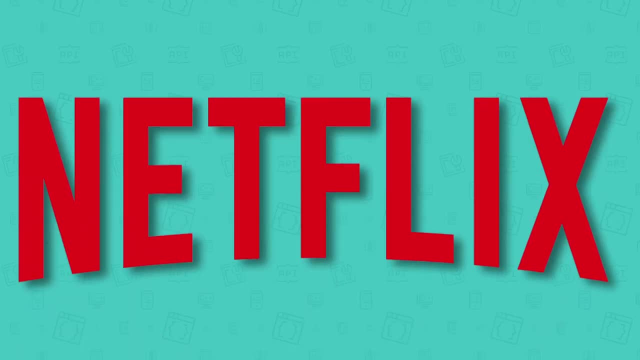 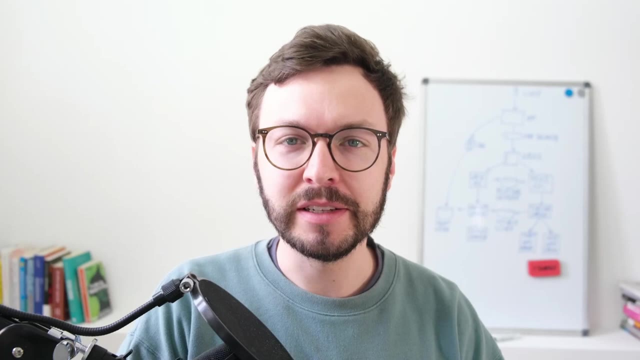 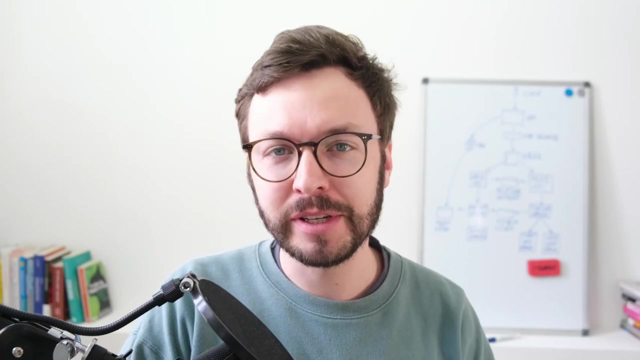 course through all the large scale systems like Netflix, YouTube, Amazon, Dropbox, Instagram, Facebook, Twitter, WhatsApp and many more. I want you to pass the interview with confidence and ease. The course was fun to watch, because learning something new shouldn't be feeling like a grind- Not at all. So if you're 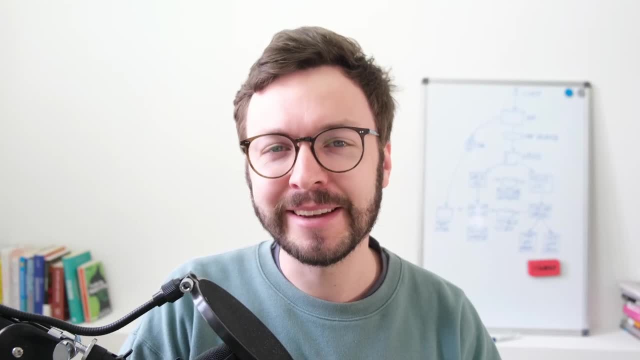 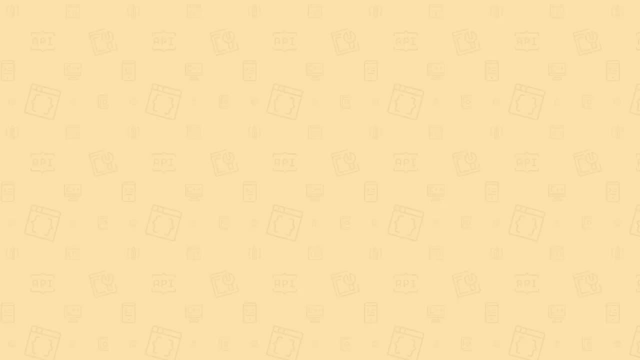 interested, just check out the link in the top right corner and again in the video description below. Thank you so much for watching this video and see you next time. Bye for now. 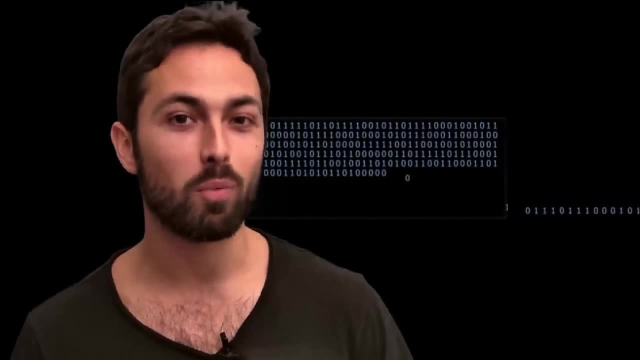 A classical computer performs operations using classical bits, which can be either 0 or 1.. Now, in contrast, a quantum computer uses quantum bits, or qubits, and they can be both 0 and 1 at the same time, And it is this that gives a quantum computer its superior computing. 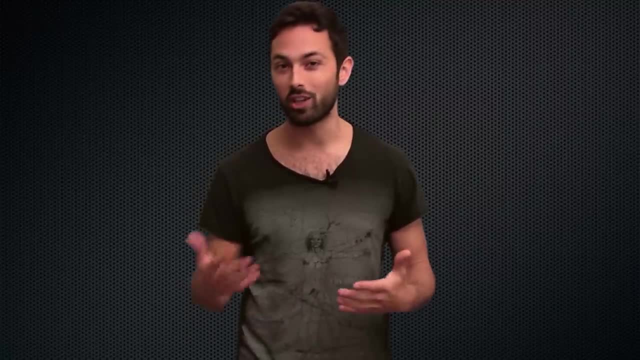 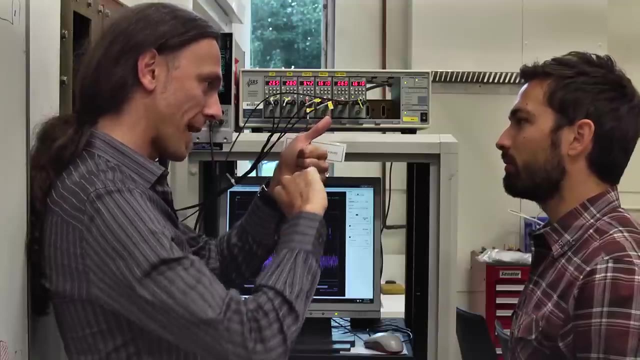 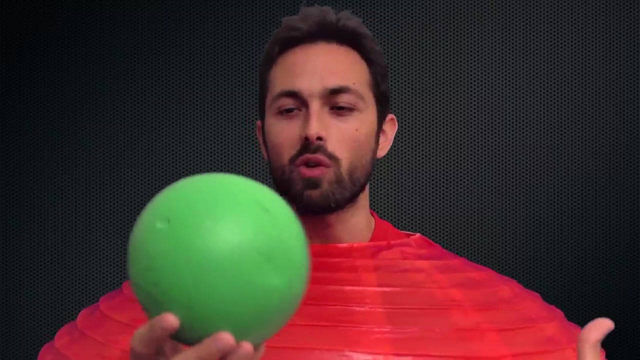 power. There are a number of physical objects that can be used as a qubit: A single photon, a nucleus or an electron. I met up with researchers who were using the outermost electron in phosphorus as a qubit. But how does that work? Well, all electrons have magnetic fields, so they're 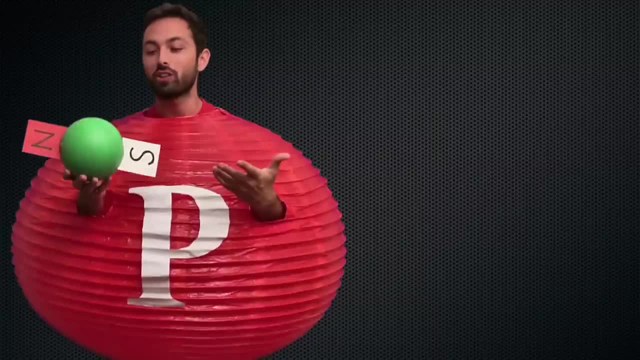 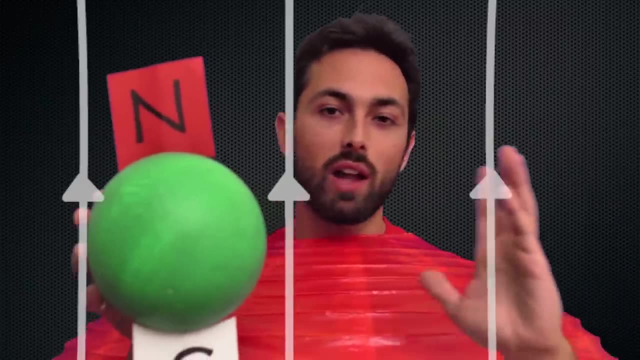 basically like tiny bar magnets, And this property is called spin. If you place them in a magnetic field, they will align with that field, just like a compass needle lines up with the magnetic field of the Earth. Now, this is the lowest energy state, so you could.